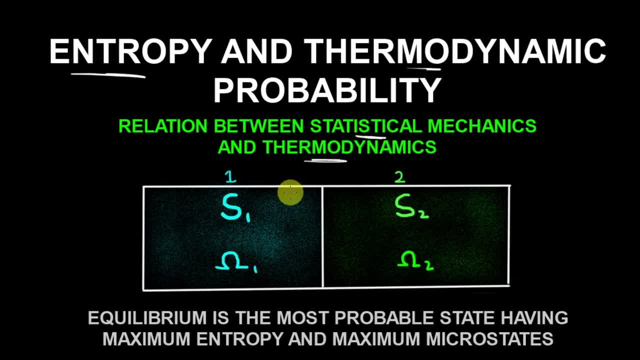 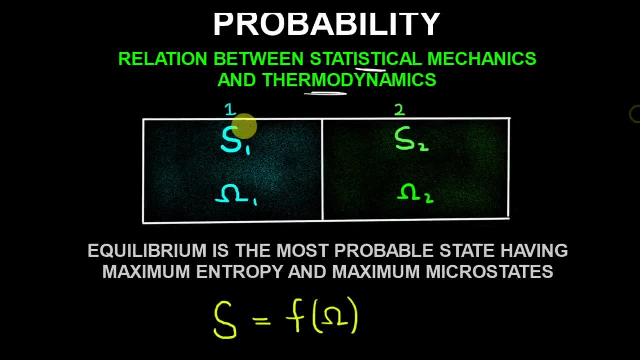 is as important as E equals mc square in relativity. So this is a really important relation. So let us derive that. Let us take two independent systems, System number 1 and system number 2.. The entropy of system number 1 is S1 and the entropy of system number 2 is S2.. The number of microstates: 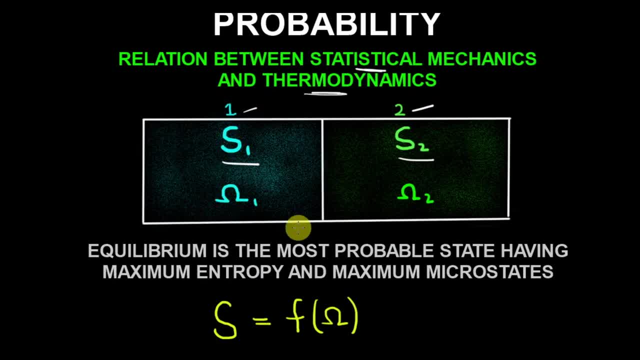 that means the thermodynamic probability of system number 1 is omega 1 and for system number 2, it is omega 2.. Now, as we know that equilibrium is the most probable state, that means a system always tends toward equilibrium have the maximum entropy and the maximum number of microstates. 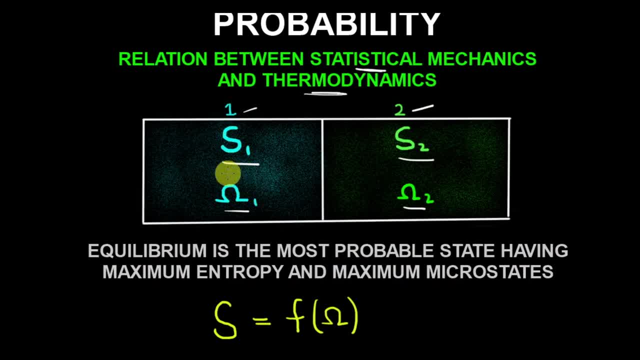 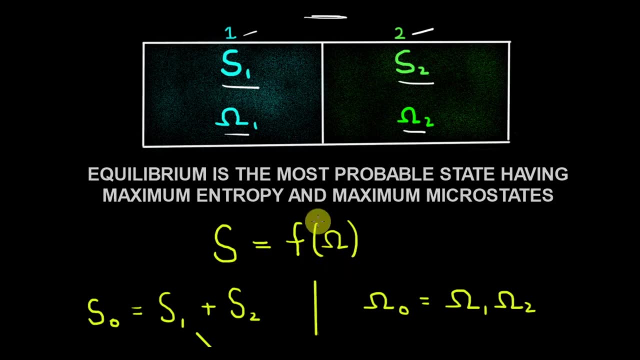 So this means that this entropy and thermodynamic probability- that means the number of microstates- is somehow related. So the entropy is the function of thermodynamic probability, that means the number of microstates. So S is some function of omega. Now, as we know, 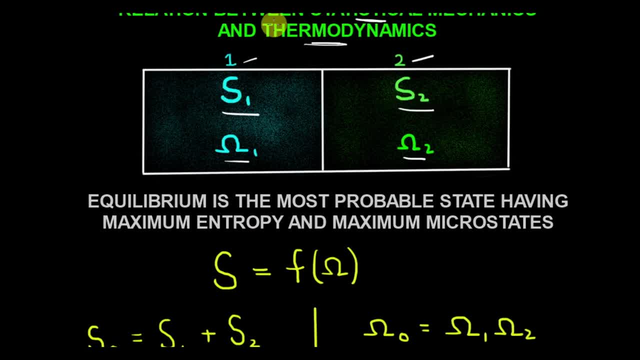 that entropy is an extensive variable. that means it's additive. So the total entropy of this system is S1 plus S2, not like temperature, like if temperature here is 300 Kelvin and it here is 300 Kelvin and the total is 600 Kelvin. No, temperature is an intensive property, It is 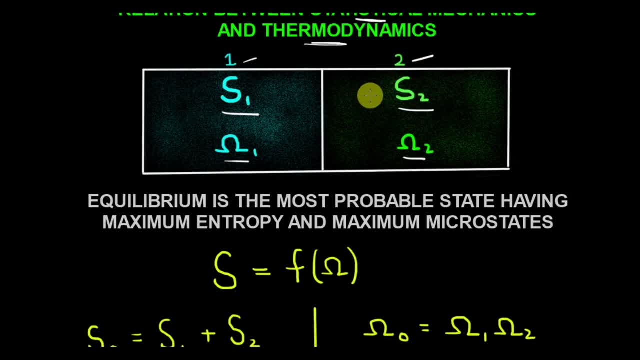 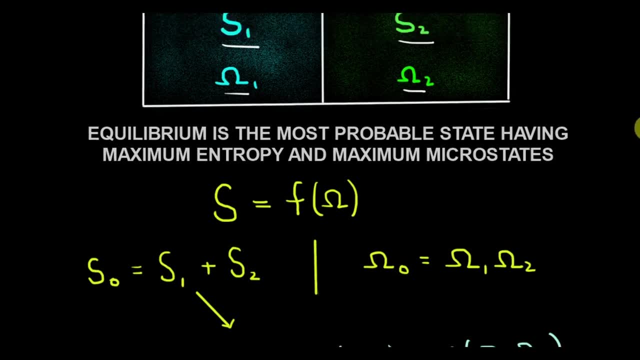 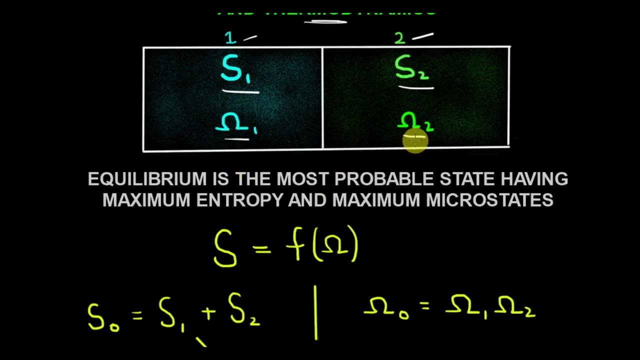 not additive. but entropy is an extensive property, So it is additive. So the total entropy of this system is S1 plus S2.. Now see this: The total number of microstates of this whole system is equal to omega 1 times omega 2.. This 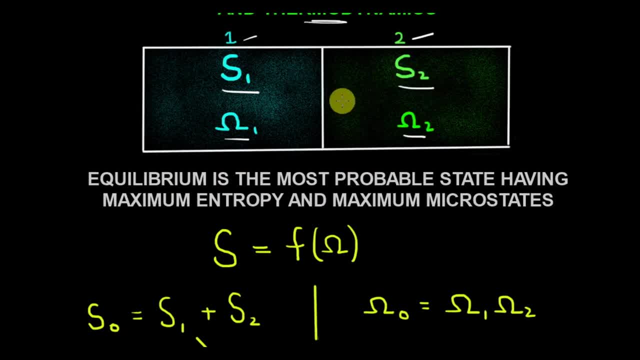 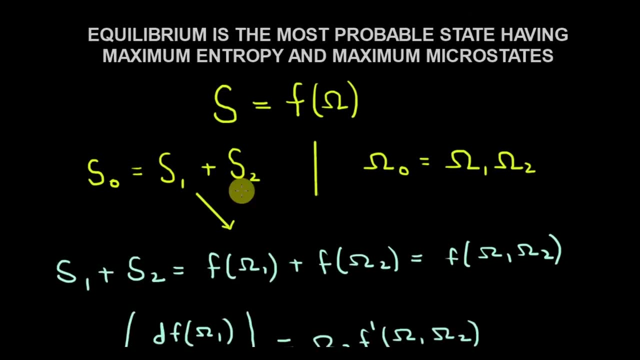 is because for each microstate of this system there should be omega 1 microstates of this system. So the total number of microstate of this system, number 1 plus system number 2, is omega 1 times omega 2.. So now this S1 is some function of omega 1 and this S2 is some function of omega 2.. 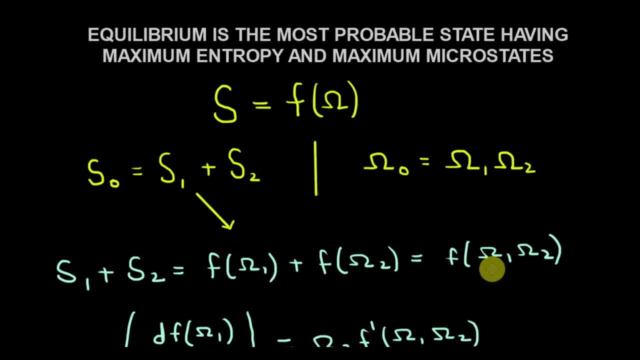 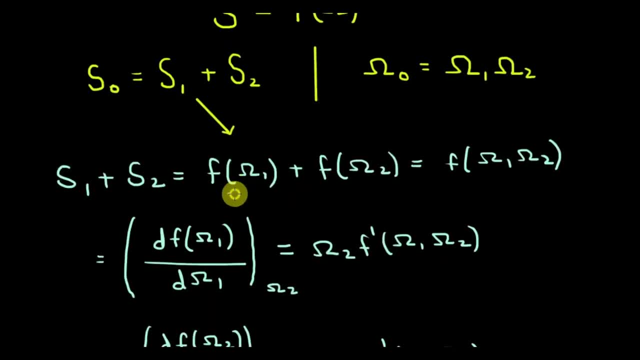 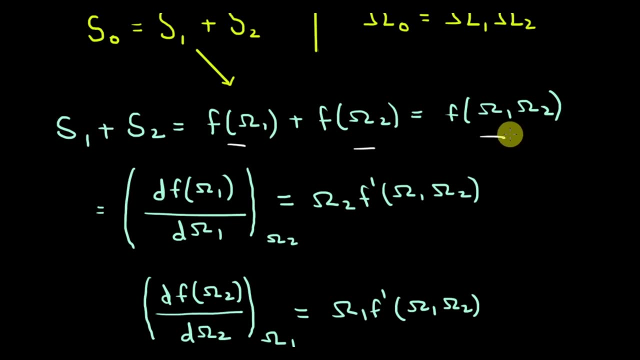 And the total entropy S0 is some function of omega 1 times omega 2.. So this is our relation, that we need this one. okay, Now we will do a simple thing: We will derivative this relation with respect to omega 1.. We will do a partial derivative. 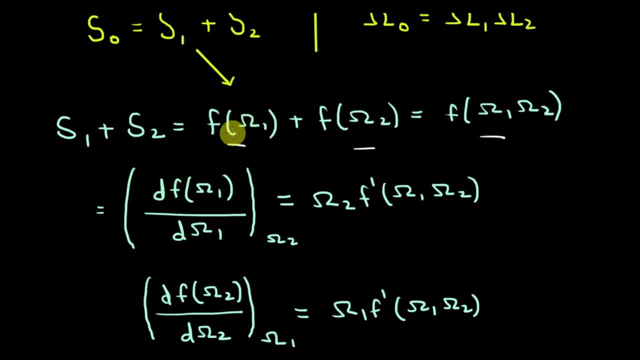 but here I have written a total derivative because this one is just a function of omega1.. So partial derivative changes to a derivative: S0 1 times S2 becomes omega1 plus omega2.. total derivative, So derivative of this function with respect to omega 1 and the derivative of this. 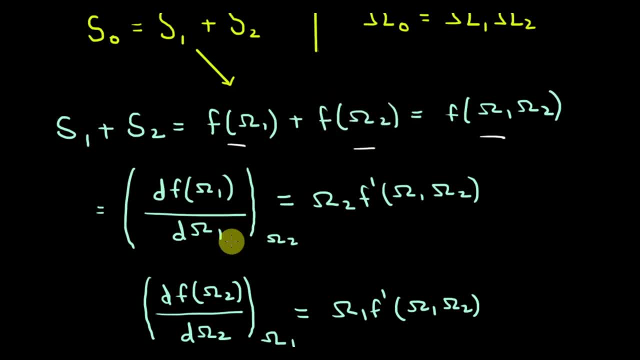 function with respect to omega 1 is 0, because this function is not a function of this omega 1 and I have written this omega 2, which is constant, which is equal to now derivative of this function, which is f dash times omega 1- omega 2.. This f? dash means df- omega 1, omega 2 divided by d omega 1. 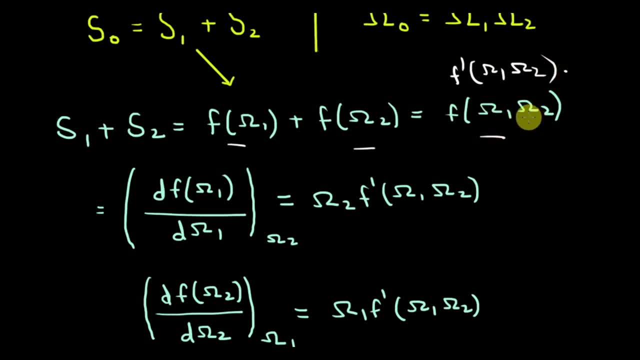 times. we will use chain rule. this omega 1 times omega 2 will also be needed to differentiate it with respect to omega 1.. So d omega 1 times omega 2, divided by d omega 1 is omega 2.. So 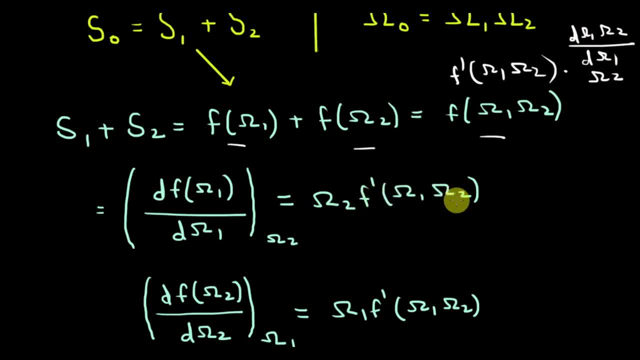 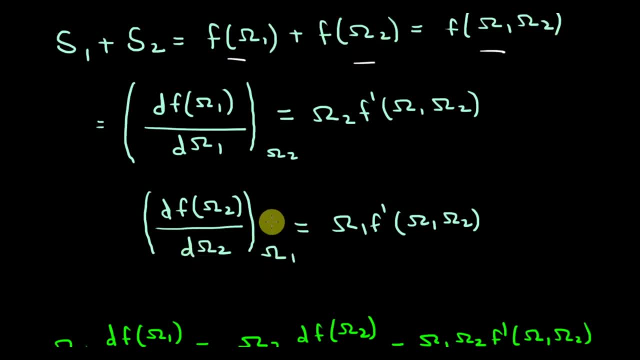 omega 2 times f, dash omega 1 times omega 2.. Now, similarly, we will differentiate this expression with respect to omega 2, keeping omega 1 constant. So this term will be 0 and we will left with df omega 2.. 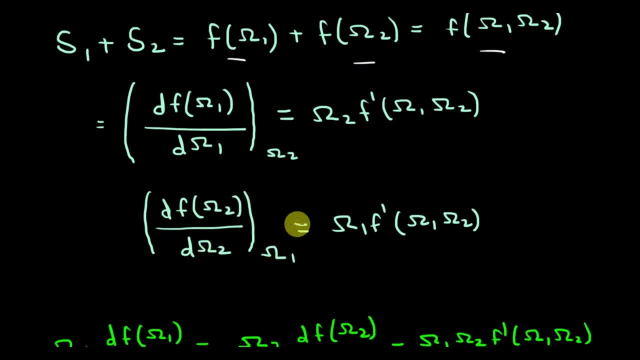 So d omega 1 times omega 2, divided by d omega 2, keeping this omega 1 constant, which is equal to, similarly derivative of this, f dash omega 1 times omega 2 with this omega 1, because derivative of this with respect to omega 2 is omega 1.. So now we have these expression, Now what we will do is 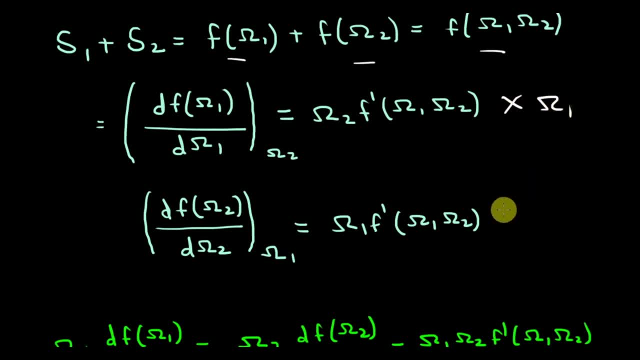 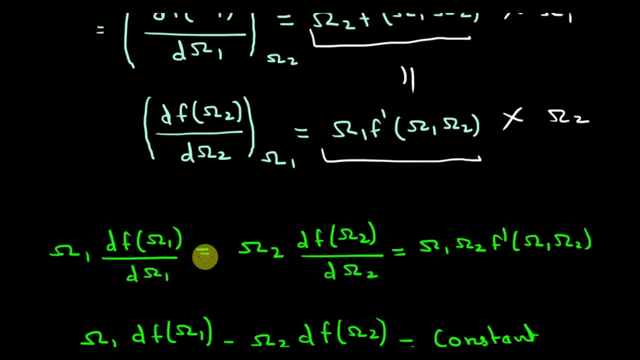 this: we will multiply this expression with omega 1 and this expression with omega 2.. So these two sides will become equal. We will released this and we will have this: that omega 1 times df, omega 1 by d, omega 1 is equal to: 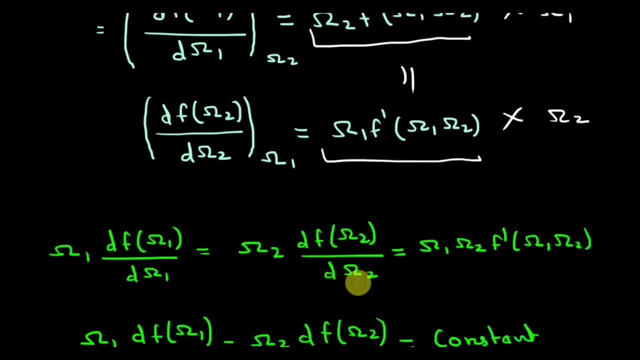 omega 2, df omega 2 by d omega 2, which is equal to omega 1 times omega 2, this thing f dash omega 1 times omega 2.. Now see this in here. this one is a function totally of omega 1.. This one, 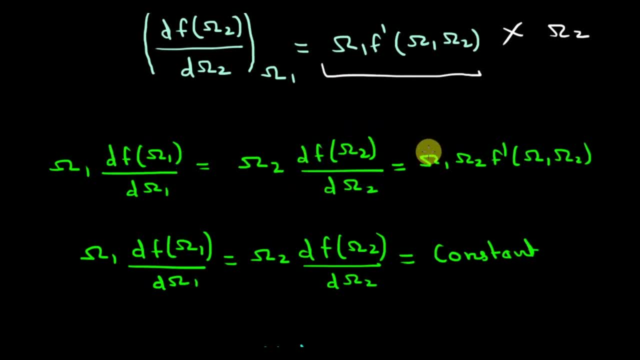 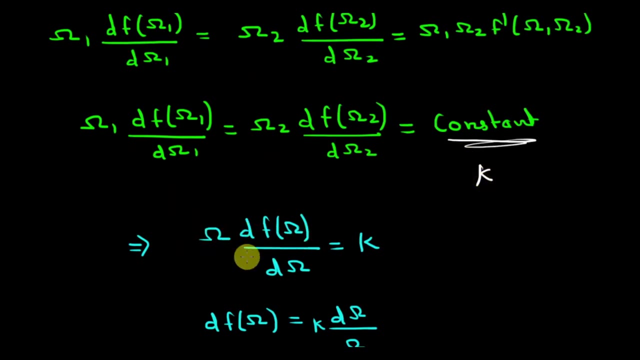 is a function of totally omega 2, and this in here has omega 1 and omega 2.. So this must be a constant, So this is equal to constant. Now let's write this constant as k, So in generally we can write omega, df, omega by d. omega is equal to some constant k. 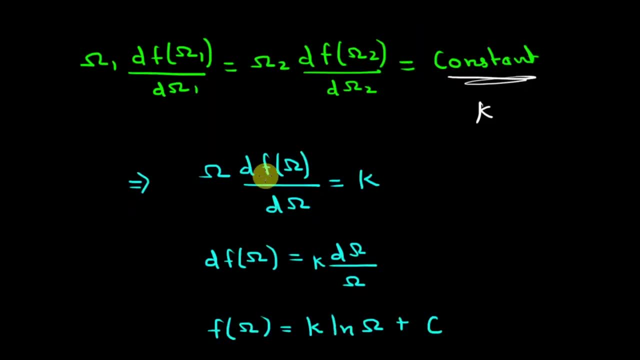 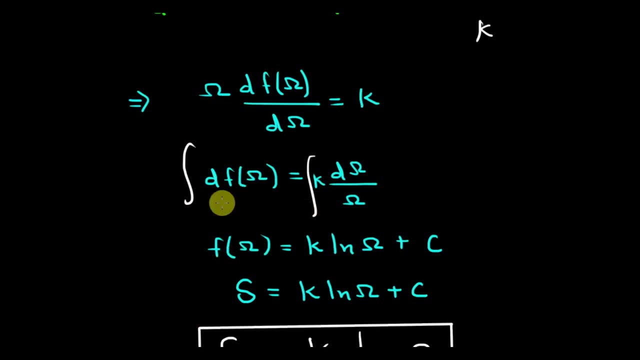 Now taking this d omega in here and omega in here and then integrating this thing, We have f omega. integration of df omega is f omega and integration of one upon omega. That means integration of one upon x. dx is log of x and this k is a constant. 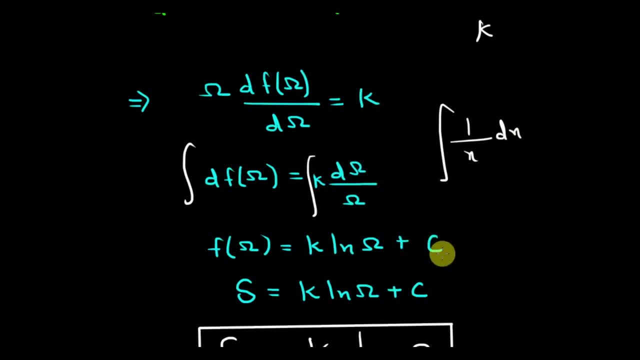 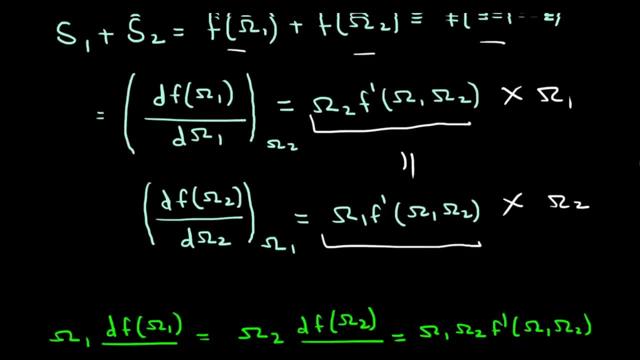 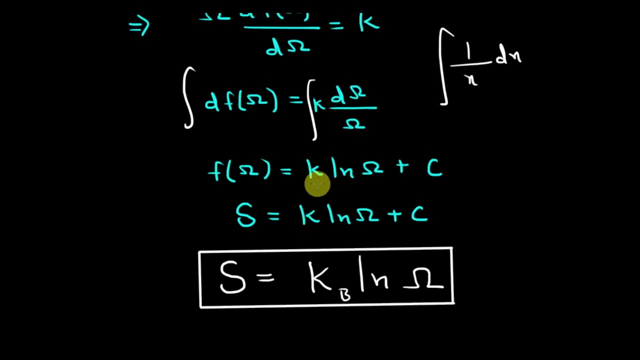 So constant times, the integration plus some constant c, which is the integration constant. Now this f omega is, simply see this entropy. So we will write f omega as entropy, which is equal to k ln of omega plus c. 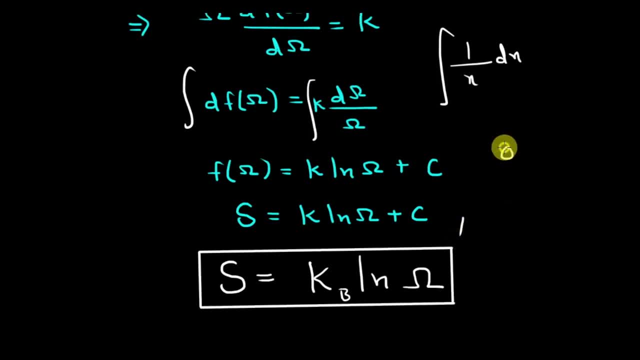 Now see this: At z, This is zero kelvin, The entropy is zero and the number of microstates is one. That means the system is like set in one state, So ln of one is zero, So c is zero. 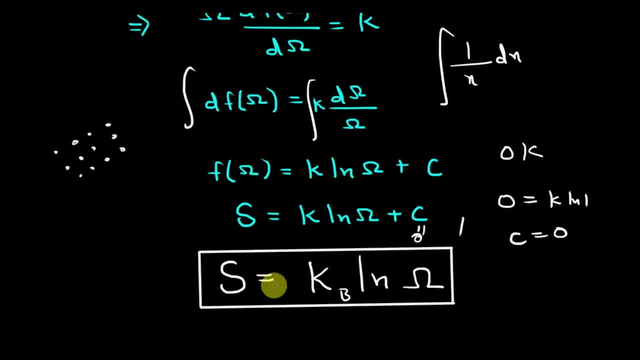 So this constant is simply zero. So we have this relation: s is equal to k, ln of omega, And this k turns out to be a Boltzmann constant, which is kb. So this relation is a relationship between entropy and thermodynamic probability, which 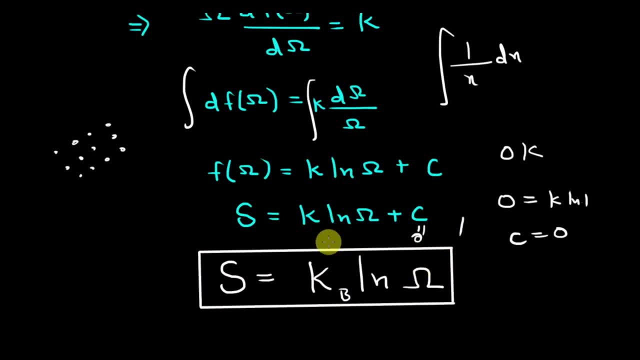 is the number of microstates. So this relation is the relationship between thermodynamics and statistics. So this is a really important relation. So I hope you have learned how to derive this relation. If you have any questions, you can ask in the comment section below. 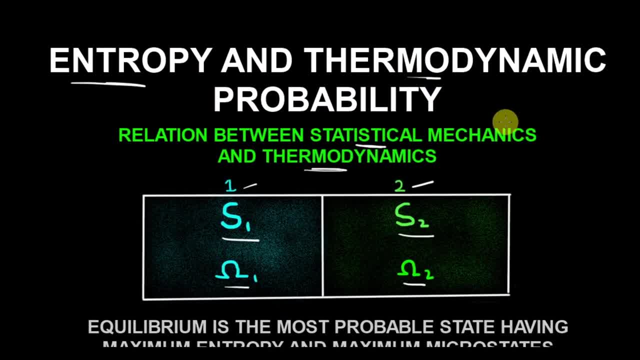 Thanks for watching this video and subscribe this channel for more videos like this one.